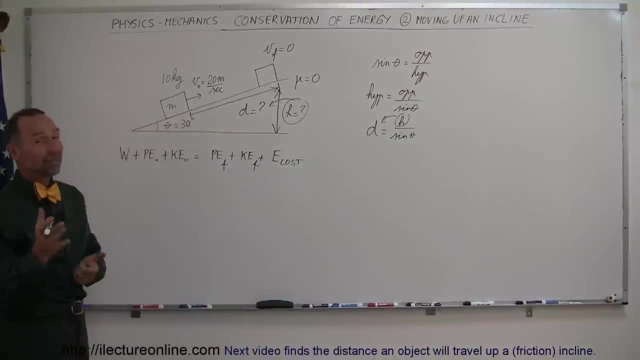 So we always put down that equation. Now the next step is to figure out which ones of these we don't have. We don't have any work input Now we can do, because we have to do something to get the object moving at 20 meters per second. but that's not part of the problem. 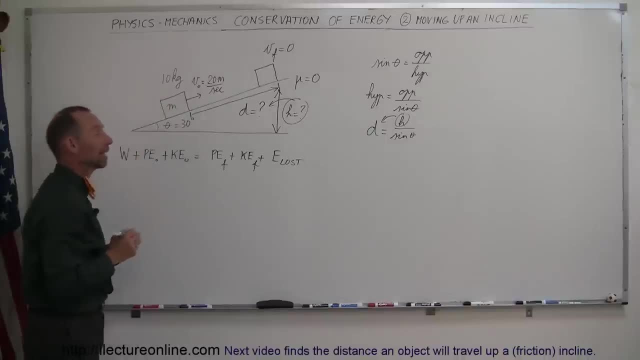 We already take that into account by saying it has this much kinetic energy. Once we give that block a push, we don't keep pushing it up the incline, so we don't put any additional work into the system. So work put into the system is zero. 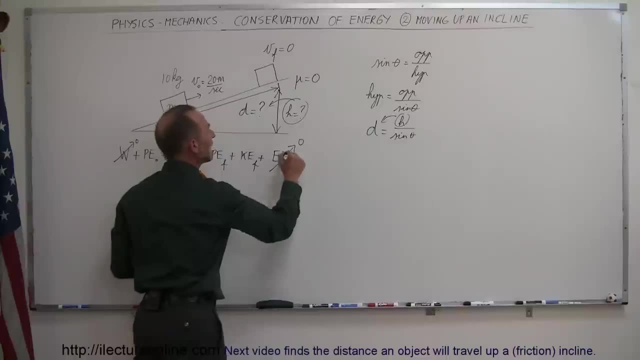 They told us that there's no friction, so therefore there's not going to be any energy lost during the process. We're also told that when it gets to the very top here, the final velocity is zero and it has no velocity. 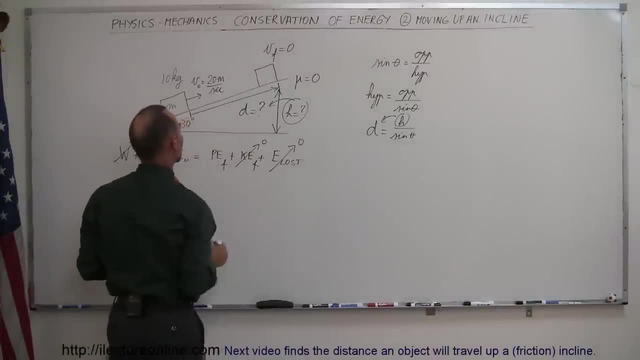 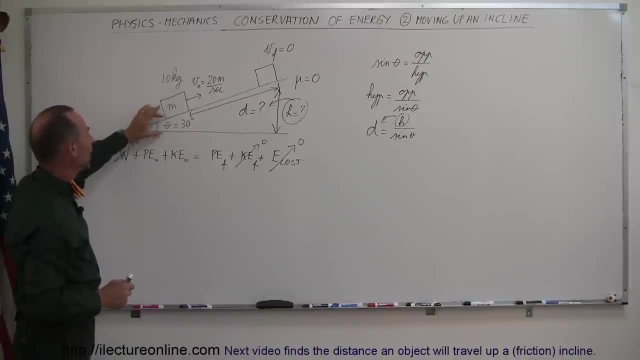 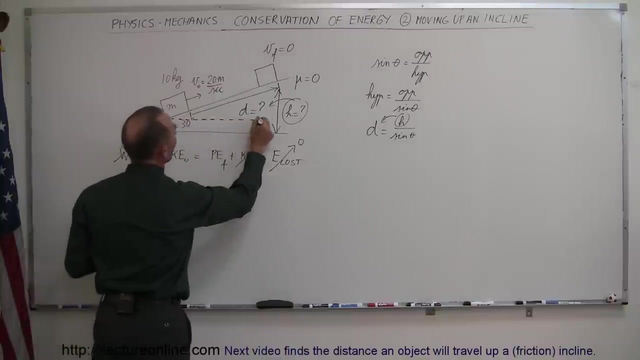 that means it has no kinetic energy. so that goes to zero as well. And here's one more trick: Even though the block appears to be starting at some initial height above the ground, we can just arbitrarily call that zero height And get rid of that. we can call this the increase in height. 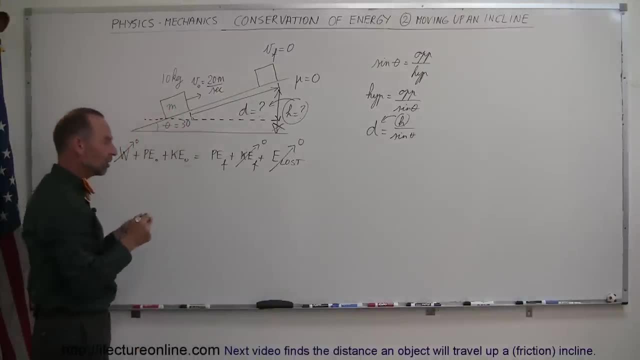 and so therefore, we can assume that it has no potential energy when it started. So we can arbitrarily put the zero height at any place that we want to make it convenient for the problem. So therefore, in this case, we can say that we have no initial potential energy. 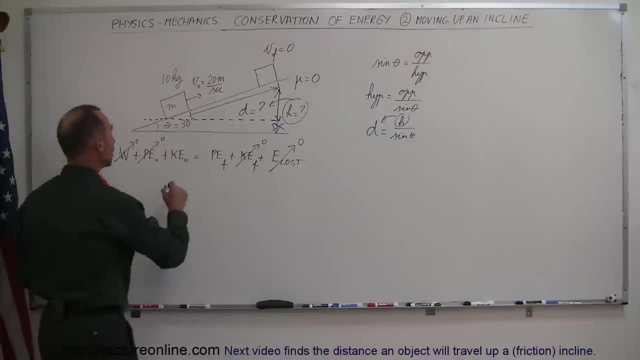 And then this whole equation simply boils down to: the initial kinetic energy is equal to the final potential energy, And, of course, the initial kinetic energy is equal to one-half mv initial squared, and the final potential energy is mgh. final. 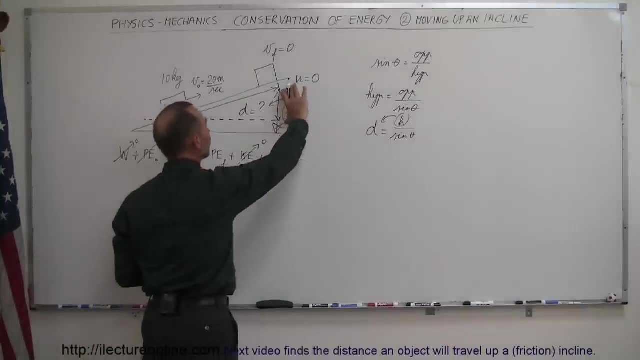 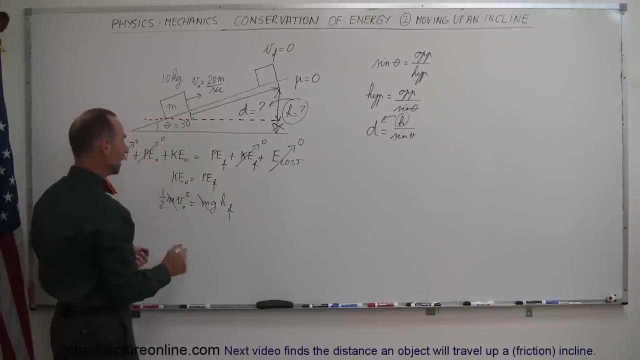 So what are we looking for now? We're looking for this Increase in height. We're looking for h. That means we want to divide both sides by mg. Now, first, I can go ahead and divide both sides by m. 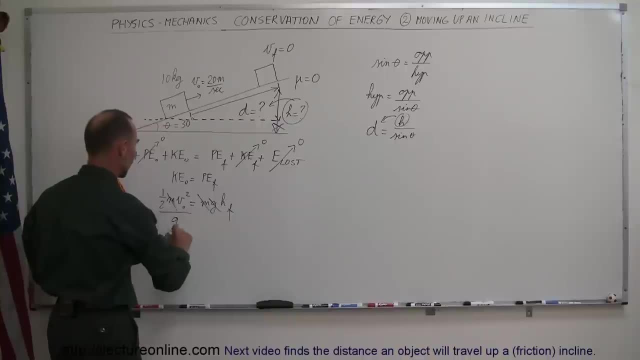 And then if I divide both sides by g, this comes over here And I can write this as h final is equal to one-half the initial velocity squared divided by g. If I plug in the numbers, I get one-half times the initial velocity, which is 20 meters per second. 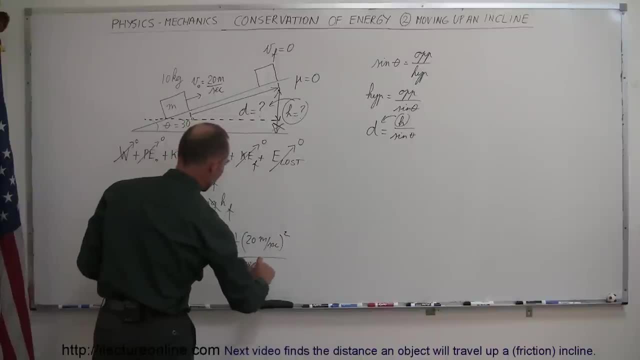 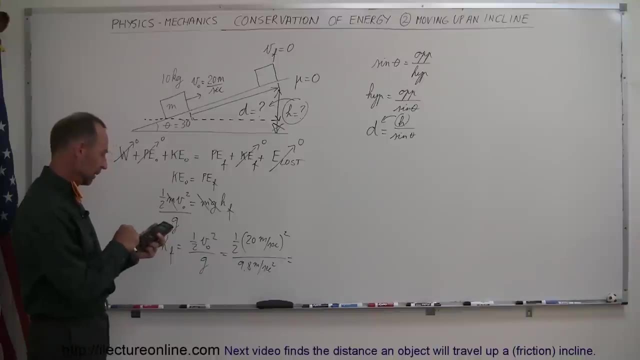 And I can square that, divide it by g, which is 9.8 meters per second squared, And that will give us the final height. So that gives us 400 divided by 2 and divided by 9.8.. 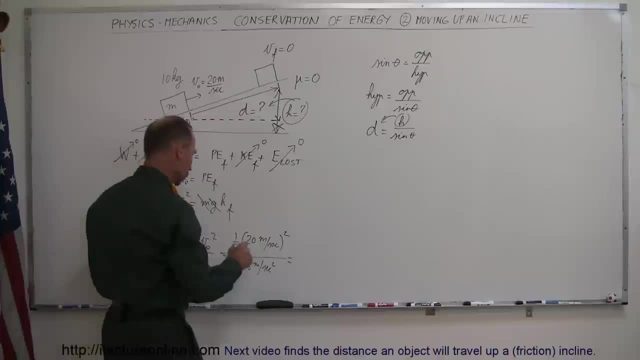 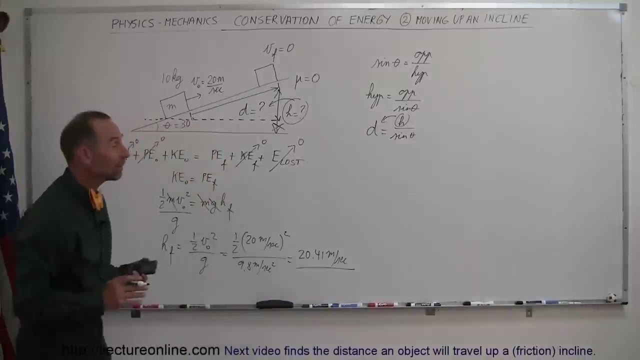 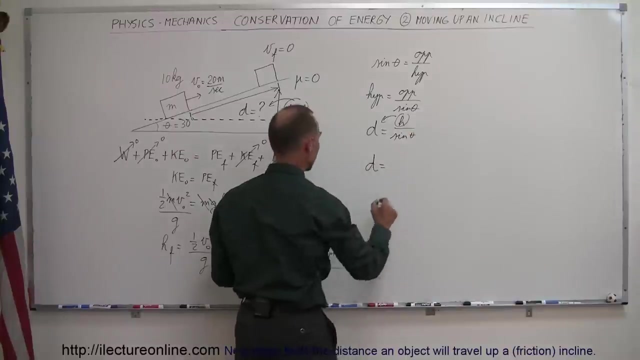 That gives us 20.41 meters per second. All right, that's how much height it gained, But that's not how far it traveled up the incline. For that we need to plug that number in here. So the distance is equal to. 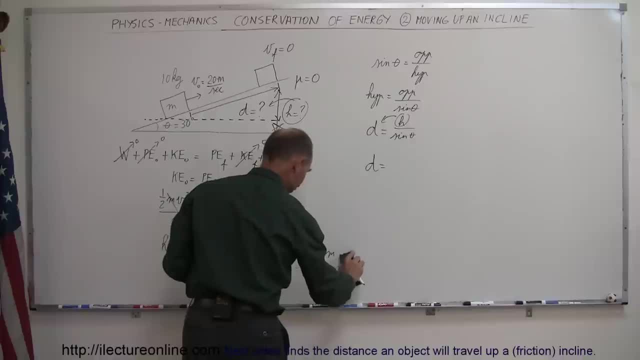 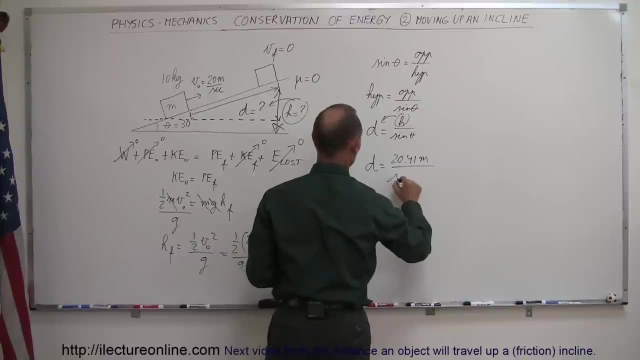 Oh, it's not 20.. It's not per second, It's height, It's just 20.41 meters. So 20.41 meters divided by the sine of 30 degrees, And of course the sine of 30 degrees is one-half. 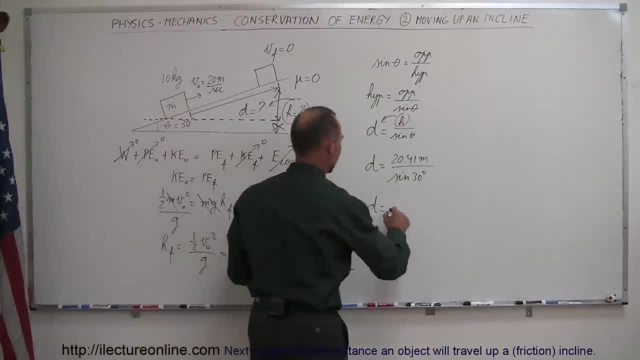 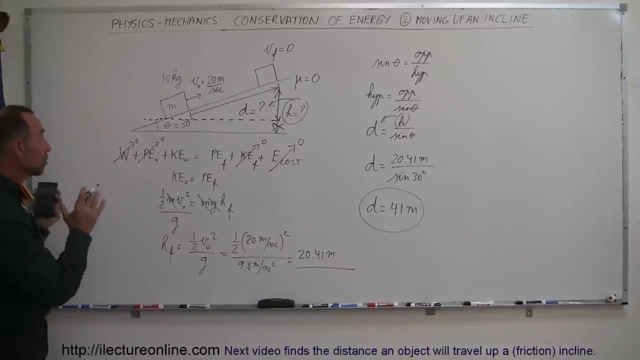 So it's like doubling that times 2. And roughly it goes a distance of 41 meters before coming to a stop. So notice how easy that problem becomes when you use that equation like that. Might as well use all the potential. 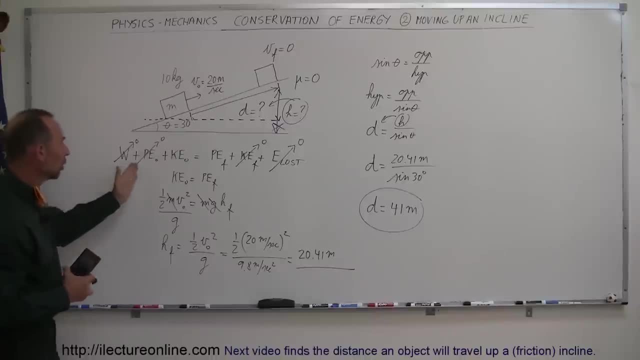 terms that could be in that equation. Put in all the potential terms that could have a value in the problem, Then get rid of the ones that do not And whatever is left over. solve that for the unknown variable, which in this case was the final height. 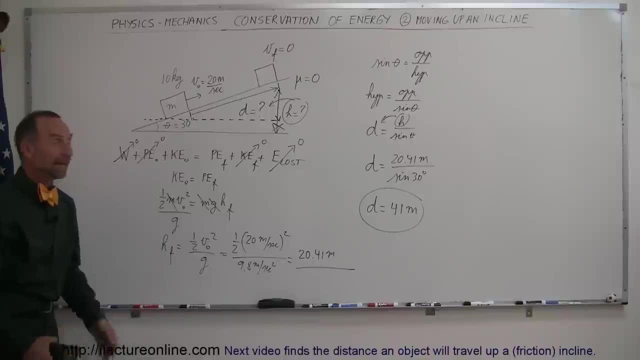 which then is used to find the distance traveled up the incline, And that's how you do a problem like that. 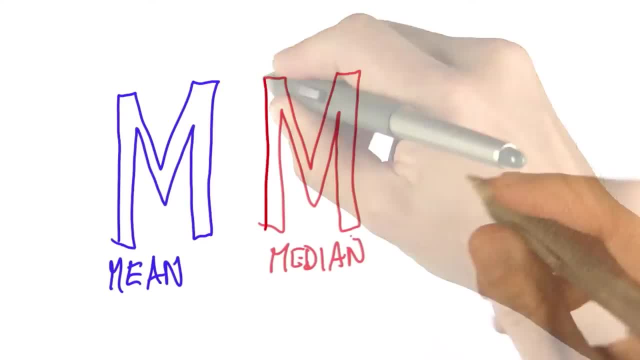 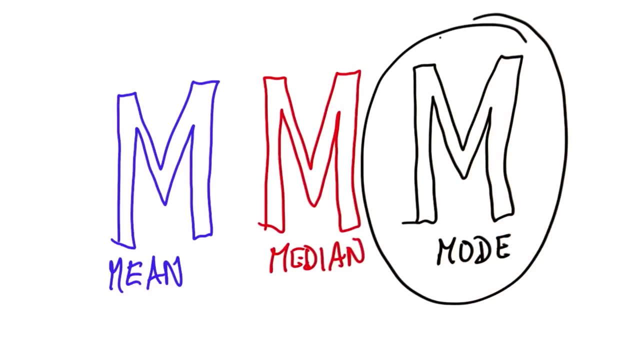 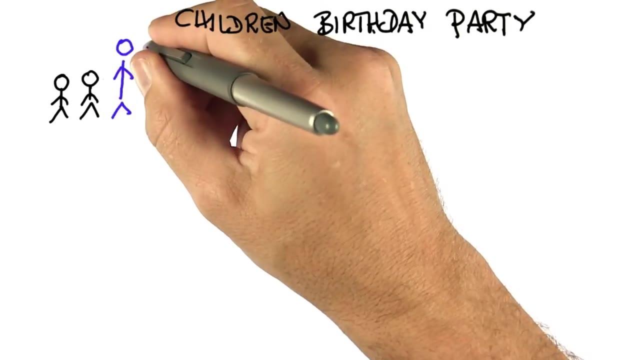 So if you learned about two of the 3Ms, the mean the median, but not the third. So let's focus on the third, the mode, And I will use as an example a children birthday party. If you've ever been one of those, there's usually kids and some of their parents. 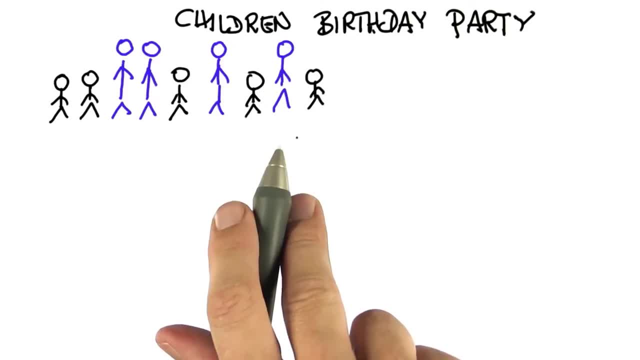 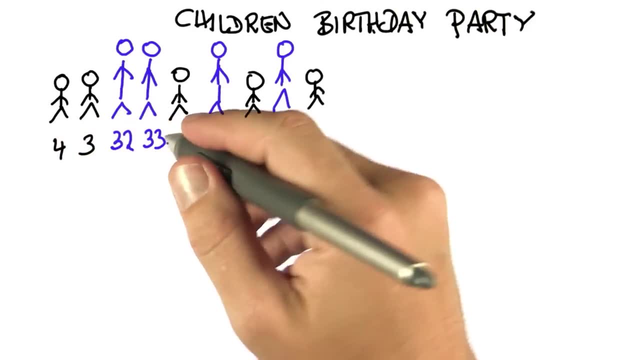 This one happens to have 5 kids and 4 parents, or 9 people in total. Let me write down the ages of the kids and the parents: 4,, 3,, 32,, 33,, 4 again, 32, again 3,, 38, and 4..